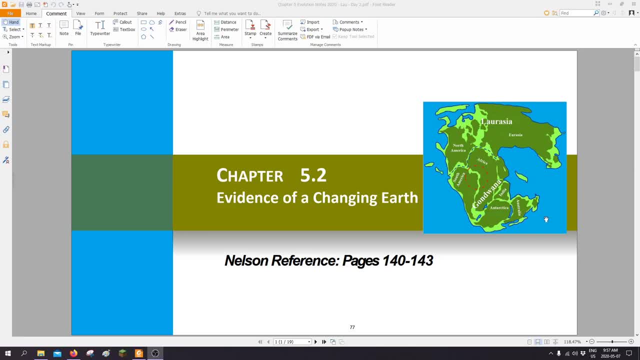 Okay, so this is going to be number two. video two: This is going to be on section 5.2 of chapter five, right? So again, we're talking about evolutionary biology: How do organisms arise into their current state, Where do they come from, etc. To do that, we're going to be taking a look at how Earth changed over time as well as how did that affect the organisms there. So this picture, this might give you a small little hint about 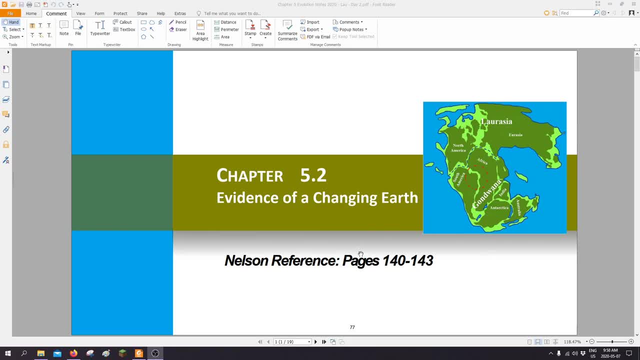 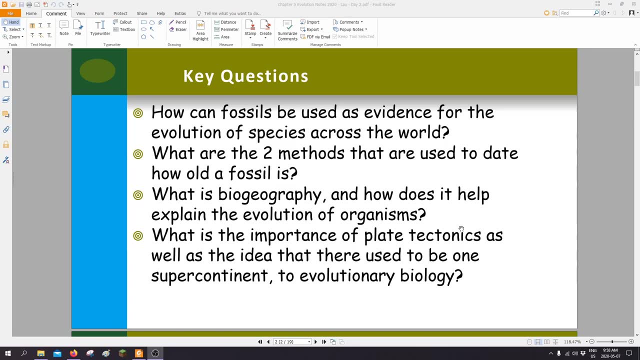 what's to come? okay, But the reference pages is going to be page 140 to 143.. Disregard the 77 there. that is an old page number, okay, So don't worry about that. Here are the key questions for this. 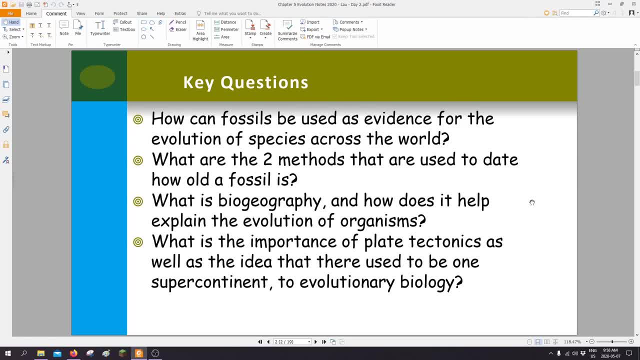 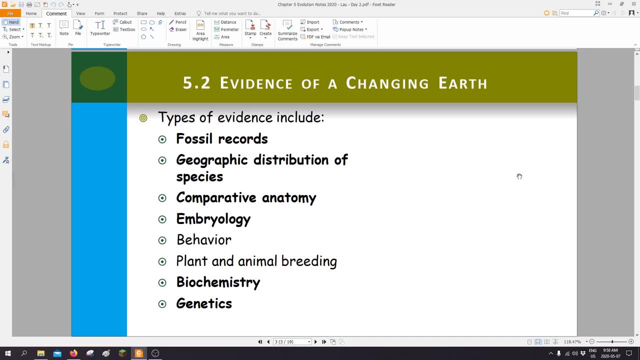 week And you can again pause this video here to take a look. All right, let's move on. So evidence of a changing Earth. So the types of evidence that we can take a look at to discover how Earth has changed over the millions of years include a few different types of evidence. 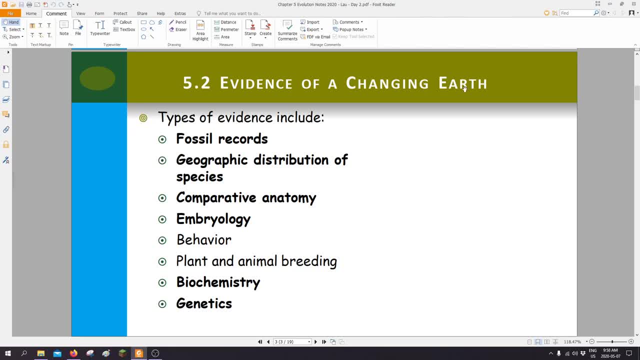 As well as sorry. this is also evidence of a changing Earth And it should also say and evidence of evolution over time. That should also be there, okay. So types of evidence for that include fossil records, geographic distribution of species, comparative anatomy, embryology. 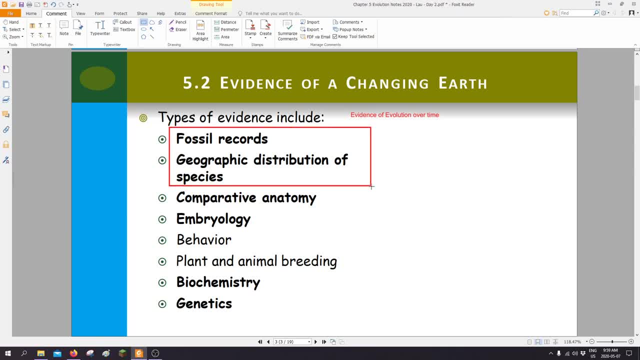 biochemistry and genetics For us. today we're going to be taking a look at these main four and then the other four that are bolded, or these main two and the other one, two, three, four that are bolded we're going to be taking a look at next week. So today we're going to be 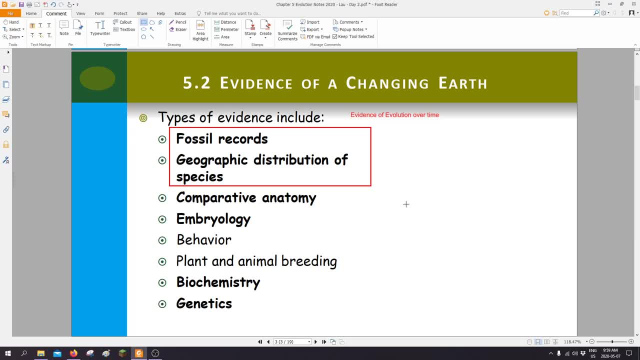 taking a look at fossil records and the geographic distribution of species. All of these, when you put it all together as an evolutionary biologist, you can then take a look at how do organisms evolve over time. So the first thing we're going to be taking a look at is the evidence from 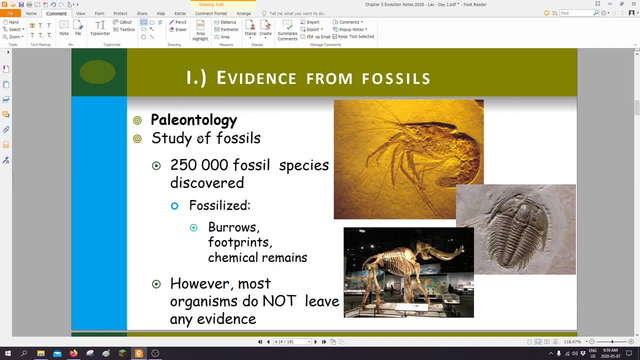 fossils. Now the study of fossils is called paleontology, and that word you may have heard it before while you were younger or if you grew up watching Jurassic Park. Now there are about 250,000 fossil species discovered- sorry- and these fossils include either burrows, footprints, 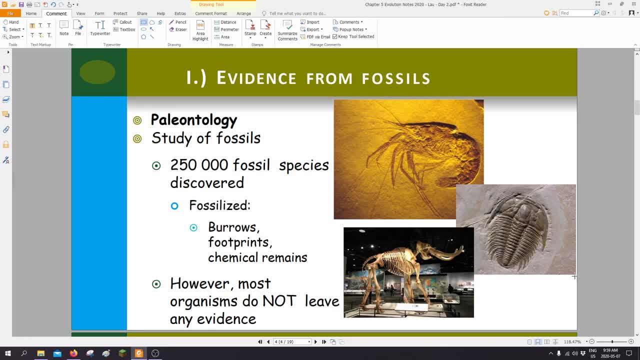 chemical remains or actual calcified fragments of the skeletons, etc. etc. etc, and also even bones and stuff. okay, Now the problem is, most organisms actually don't have any. where am I going to put it? any evidence whatsoever, okay, So you've got to be very careful about what you look at, what you use. 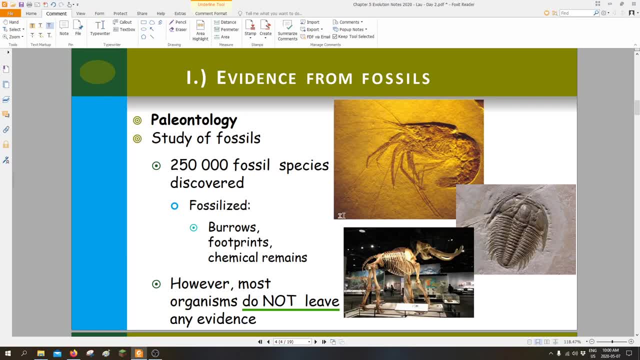 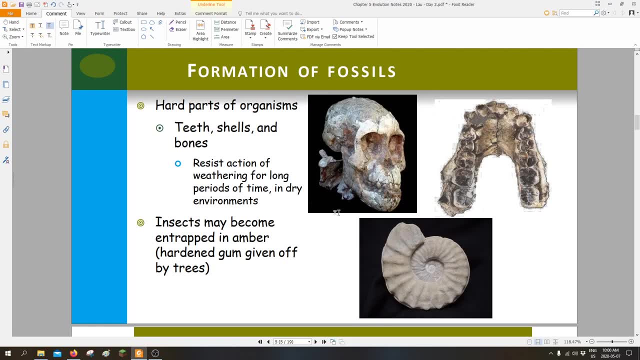 etc. to discern what is actually important and what is not. But anyways, this is the study of fossils, many different fossil types. How do fossils actually form? So a lot of the? what do you call it? What do you call it? right over here, These are bones. Wow, I'm having a. 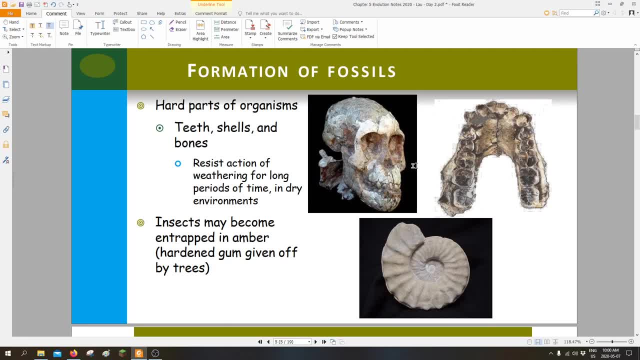 brain fart. Okay, so the hard parts of the organisms like teeth, bones, shell, etc. they degrade over time very well. They just are just preserved right in very dry environments. That's where you get fossilized teeth remains over here or bones like this or also like dinosaur bones. 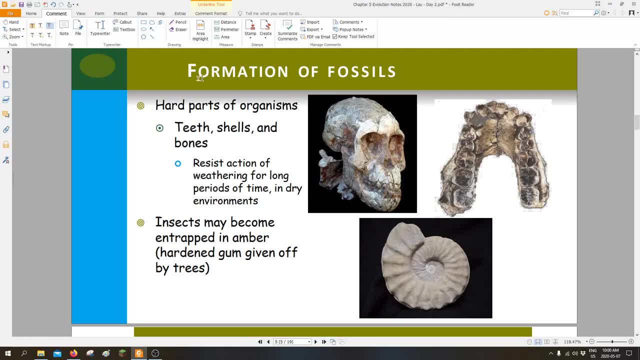 from before that also have been partly calcified as well. okay, Other ways of having the hard parts of organisms be fossilized or preserved over millions of years is, for example, insects being trapped in the amber or the hardened gum that's coming off of trees. You may have seen this in 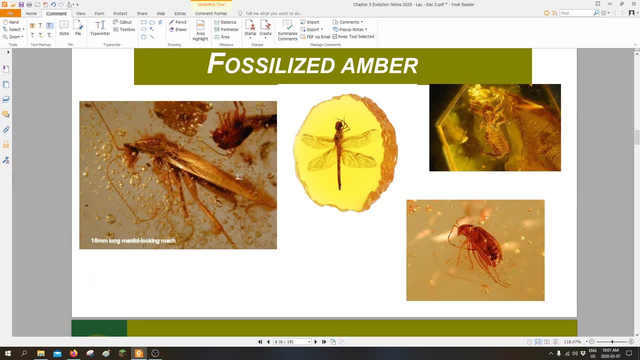 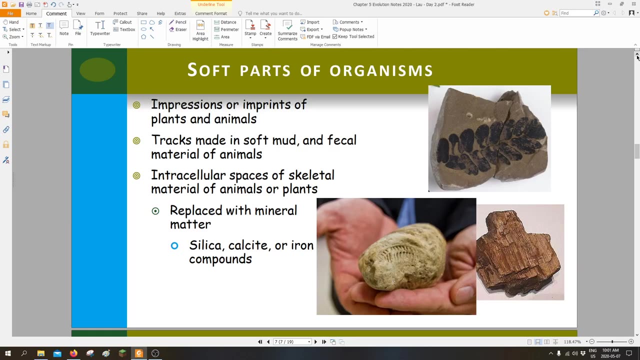 Jurassic Park, okay, where the insects get trapped in the sap and then the sap hardens over the millions of years and it just traps the insects inside, like this: now, the soft parts of organisms- these are going to be degraded over time and so they sort of just disintegrate. 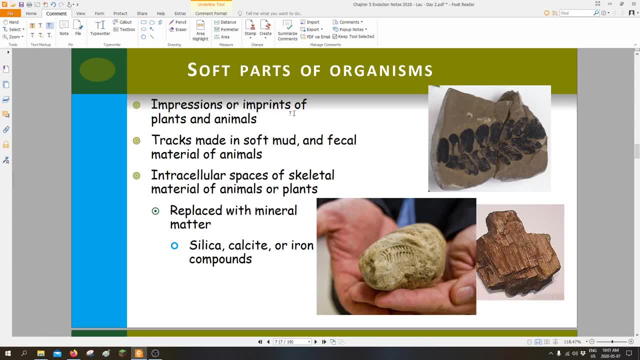 what happens is perhaps the soft parts of the organisms, like the flesh, leaves, etc. they make imprints onto stone, etc. or maybe they are made in soft mud, like the imprints, or the tracks are made in soft mud and then the tracks get filled up with um rock etc. 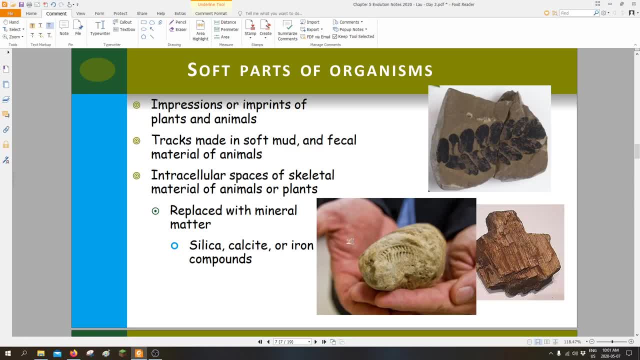 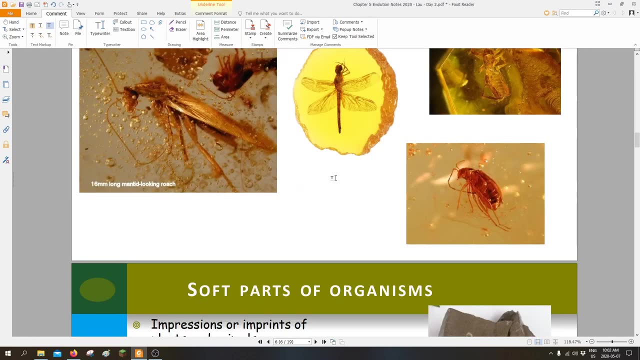 also. for example, you can even take a look at the fecal matter of animals. so fossilized poo right, that's actually a very specific um branch of paleontology specifically taking a look specifically at fossilized poo, and this is actually a sample of fossilized poo right. 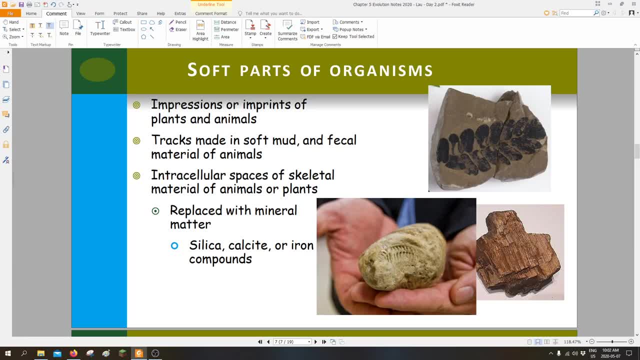 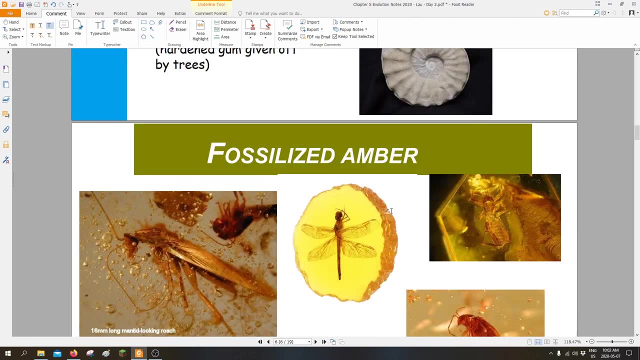 over here that has an imprint of a particular leaf in it which tells you that, oh, this is fossilized poo from an herbivore for millions of years ago. so these are the different kinds of fossils that you can take a look at: either the trapped amber insects, hardened remains or imprints. 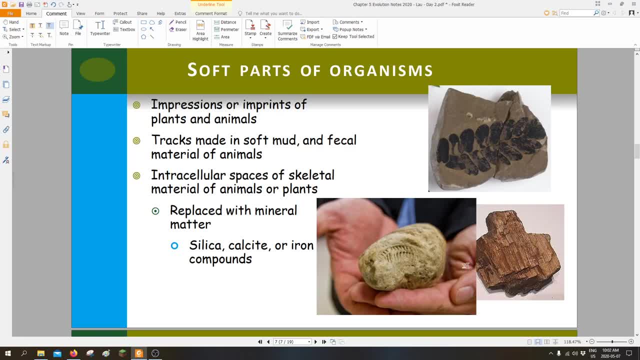 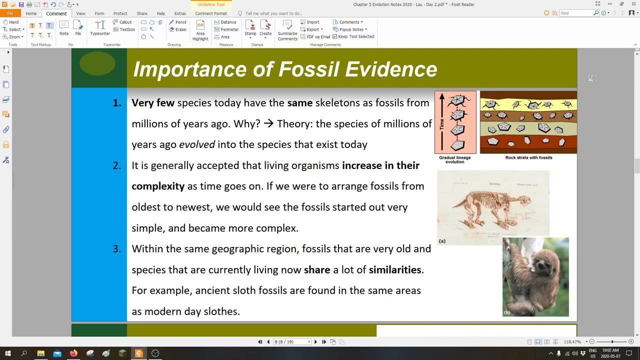 of the soft parts of the organisms there. that could also be replaced by the soft parts of the or iron compounds as the, i guess, like mud etc. the dirt go all around the different imprints or tracks. so from all these fossil evidences or pieces of fossil evidence, and we can have three main 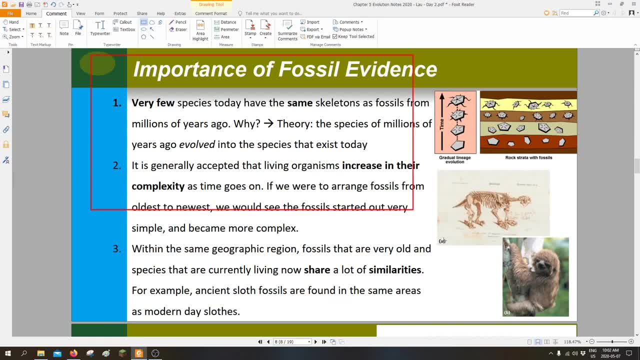 points about why fossils are actually important and all of this very, very important as to why fossils are going to be used in evolutionary biology. so the first point is number one: very few species today beingaszr. so the first point is number one: very few species today are actually working with these minerals, etc. 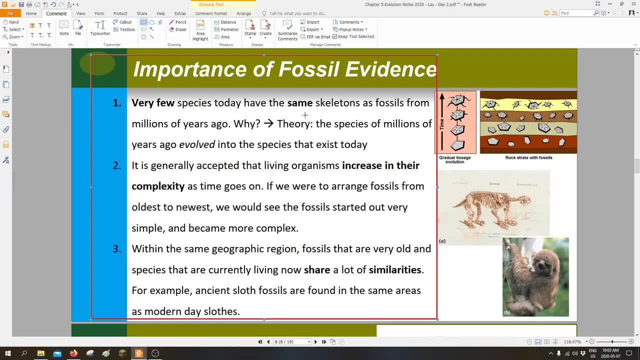 and and yourself, your journey from space. uh, producing the fossils to make it, you bring a bunch of extracts, nonsense. so the first point is number one: very few species today. but do you have to do it here? i have a little bit on this point. Number one: very few species today have the same skeletons as fossils from millions of years ago. 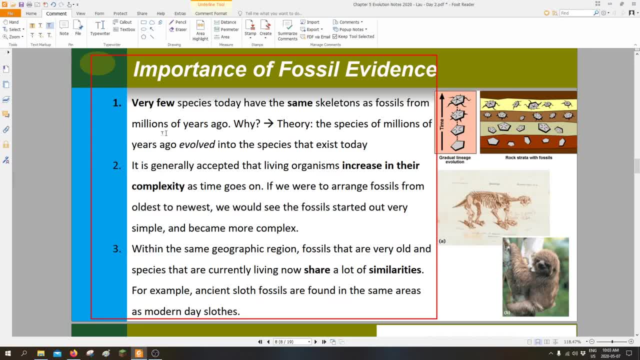 They don't have the exact same ones. Why? The species from millions of years ago evolved into the species that exist today, so their bones and skeletons naturally also change over the millions of years. So that is why fossils can be used as evidence for evolution. 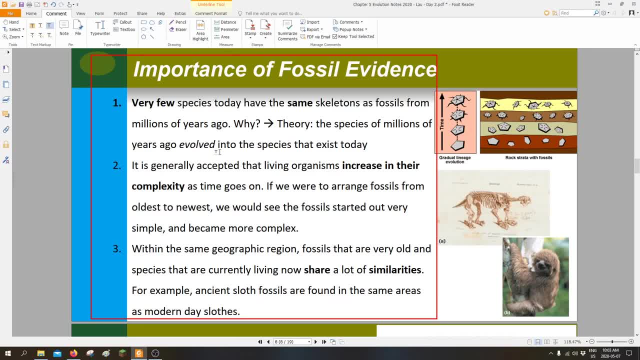 None of those animals exist now. And where do these animals that exist now come from If their bones are also not found as fossilized remains from millions of years ago before? naturally, you would think: oh, the millions of years ago these organisms and their skeletons evolved into the ones today. 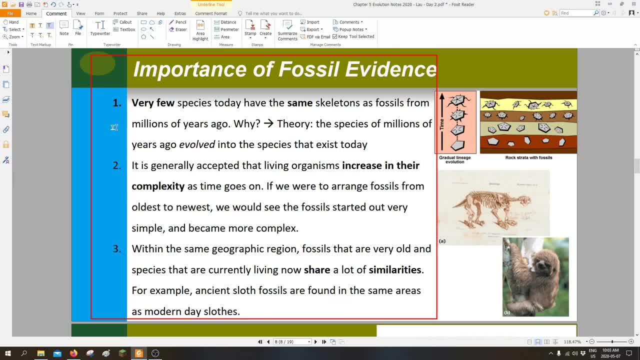 That's why we don't see any exactly the same skeletons. Number two: it's generally accepted that living organisms increase in their complexity as time goes on, and that is going to be related to this picture over here. So very, very long time ago, maybe, you would have a simple pentagon organism over here. 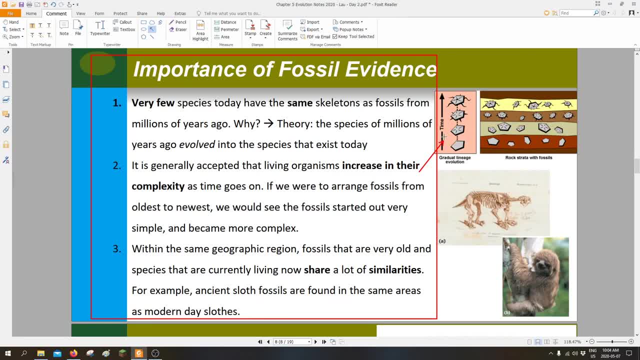 Then, as time goes on, you would have a pentagon organism over here. Then, as time goes on, you would have a pentagon organism over here. So as time goes on they get a little bit more complex over here And then at the end of it they are very complex, right. 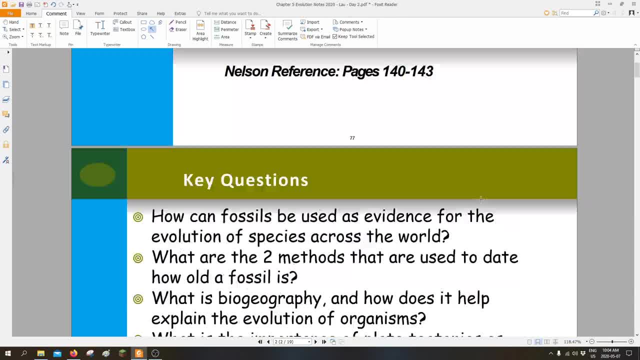 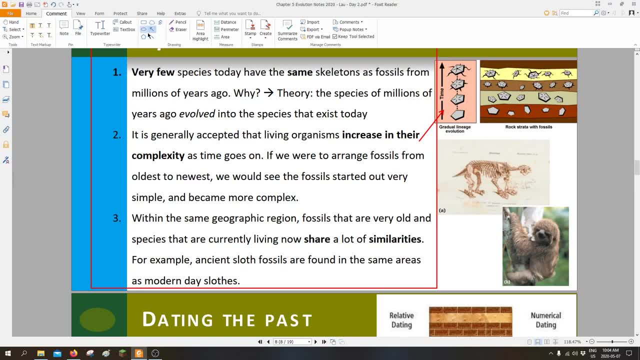 You can even think about like, for example, like, let's see, do I have a picture? Did I have? nope, not in this one, okay, But for example, like before, maybe the organisms, maybe they're just like, oh, they're just like snails or like slugs. 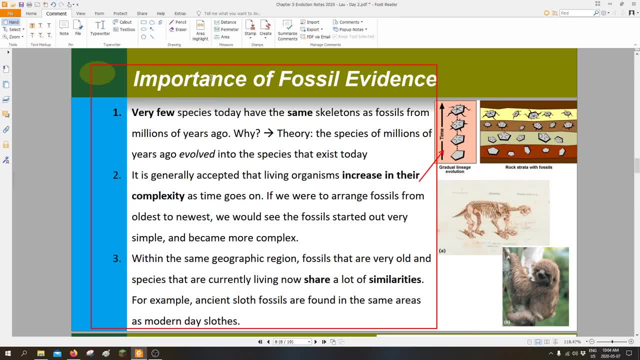 or they're just like plants and they're very, very old. And then you take a look at: oh well, you have a skeleton of them- mammal that's actually relatively young. Where did this mammal come from? Well, it is a very 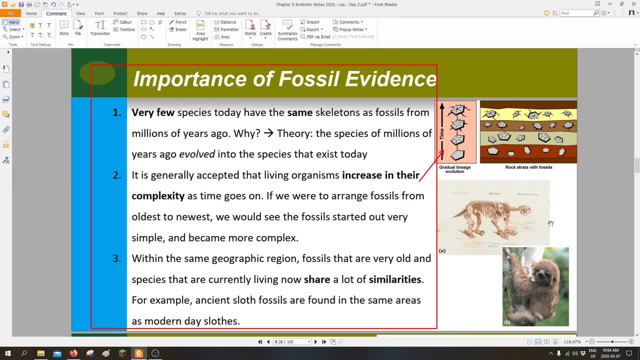 complex organism and then the simpler organisms are older. So then, if you were to arrange the fossils from oldest to newest, you would see that the fossils start out very simple and over time they become more complex or more complex. organisms start appearing as you get closer and closer to. 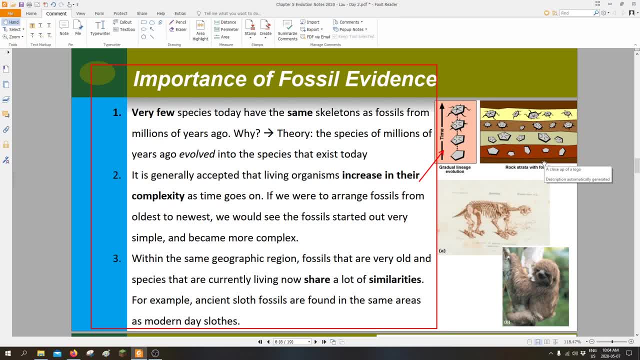 present day which tells you that okay. naturally, there must be a reason why older organisms are simple. newer organisms are more complex. Maybe it's because of evolution, or the evolution of those organisms over time. Finally, number three, which is going to be related to something called. 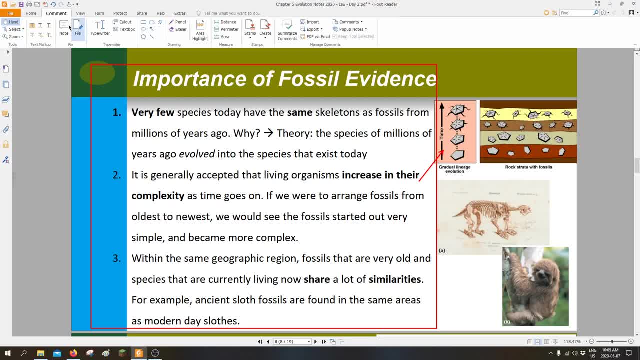 biogeography that we take a look at later on. Within the same geographic region, fossils that are very old and species that are currently living. even though their skeletons are not exactly the same, they still share a lot of similarities: For example, ancient sloths and modern day sloths. 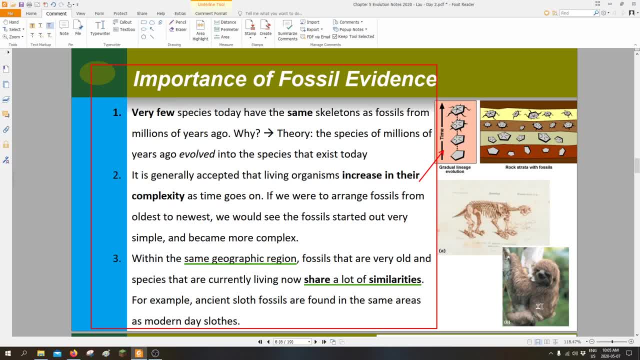 they look very similar and they're only found in the same areas, which tells us that these sloths from millions of years ago evolved into the modern day equivalents, and that is another reason why fossils are going to be very good pieces of evidence for evolution. So review number one: 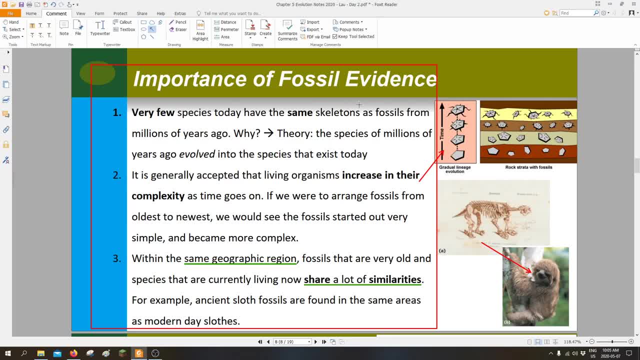 the exact same fossils are never found today and from millions of years ago, which tells us that those organisms evolved over time. Number two: if we were to arrange the fossils from oldest to newest, we see increasing complexity, which gives us a hint that evolution caused the increase in complexity. And number three: 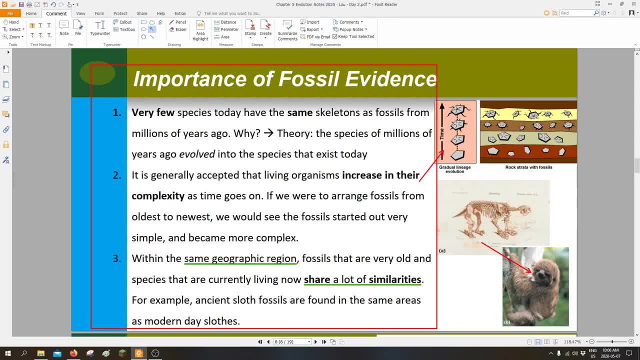 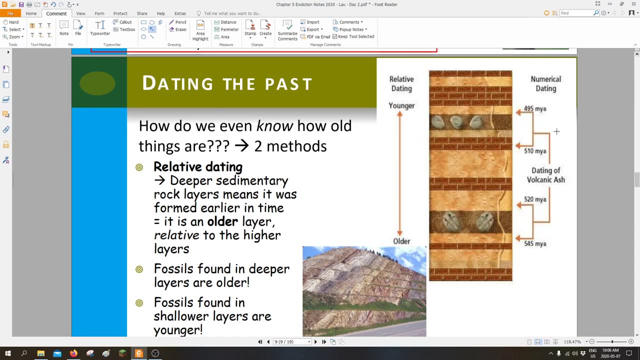 within the same geographic region. the fossils from millions of years ago have similarities to the organisms that also live in the same area, which tell us again another reason why these old organisms evolved into the new ones. Now, how exactly do we even know how old? 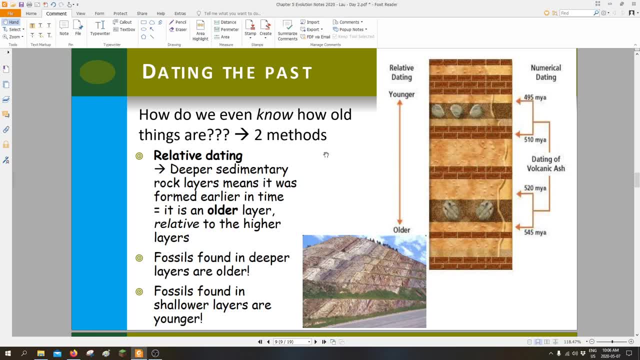 things are okay. so there are two main methods for figuring out how old fossil fossils are. okay, number one is relative dating. okay, so in the deeper, deeper layers of dirt and earth we would think, oh, deeper it is, the older it is because these layers over here they had to form on top of 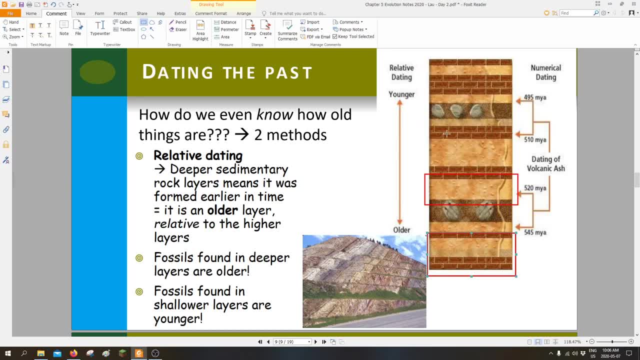 the old layers from before and these layers are covered by even newer layers. right, they didn't all appear at the same time. these layers appeared over time, okay, so, for example, like these, these layers over here would be the newest, these would be the oldest, because these top layers have to. 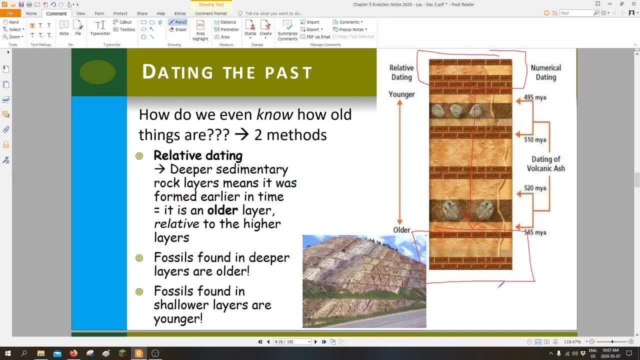 form over the old ones there. tldr: older layer is a deeper layer and deeper layers are older layers- okay. vice versa is also 어�. Onion & Flying is a deeper layer and deeper layers are older layers. okay, vice versa is also que此 true. That means over here, fossils that are found in deeper layers are older than fossils that are. 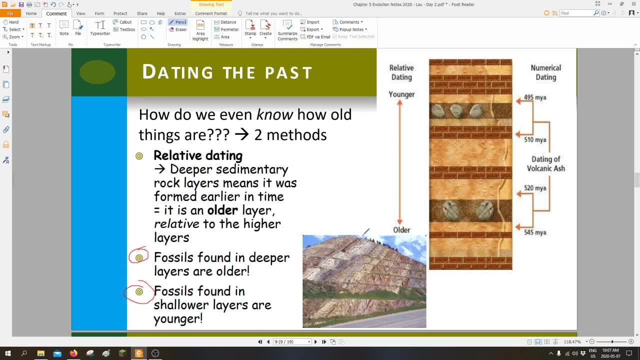 found in shallower layers. So if I found a fossil in this layer and then later on I found a fossil in this layer of the earth, fossils found deeper are going to be older and fossils found in the shallower layers are going to be younger relative to the higher layers. Now that's relative dating. 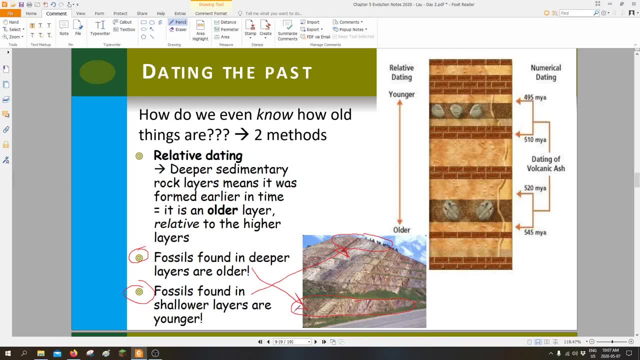 so it's not exactly the most exact. We just know that this layer on the bottom is older than the top. but just by saying the word older, that doesn't give us a number. okay, So we need a number. How do we do it? Let's take a look. Method number two is going to be called absolute dating. 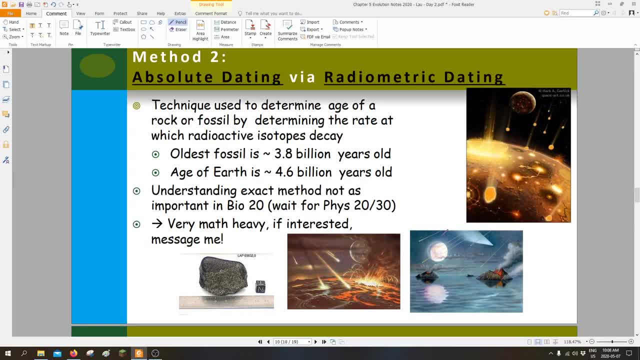 via radiometric dating. So this technique determines the number of layers that are found in the earth. So if I find a fossil in this layer and then later on I find a fossil in this layer and then later on I find a fossil in this layer, 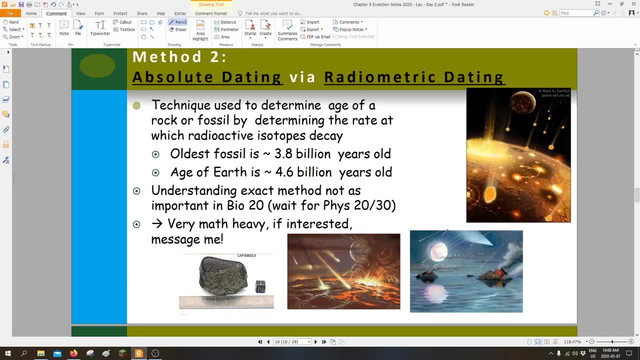 estimated exact age of the fossil by using physics as well as chemistry. So radioactive isotopes decay This section right over here. that means there are certain isotopes of elements that exist in the fossils that over a certain period of time will decay and basically just 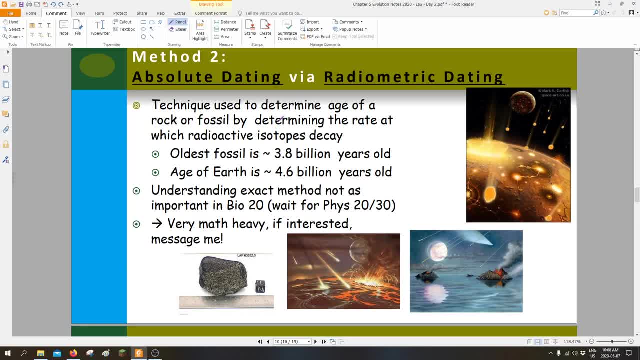 turn into other things. okay, Now I'll be honest with you right now. class right over here. understanding the exact method of radiometric dating is not very important in bio 20.. You'll learn the exact methods and how to calculate them in physics 20 and 30. However, if you're 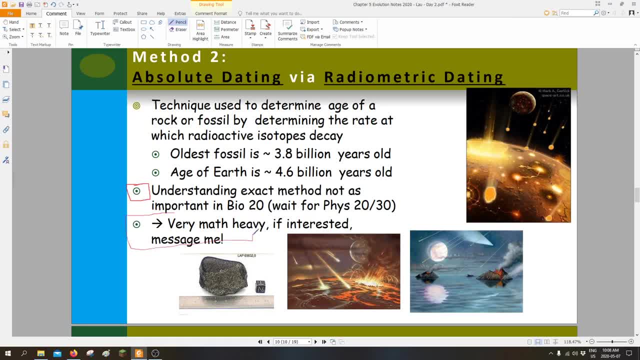 actually interested in learning how they do it. please message me. I am, oh gosh. please message me. I am prepared to explain this as best I can So you understand how the crap you figure out if something is a thousand years old or 10,000 years old, But basically by using and analyzing some 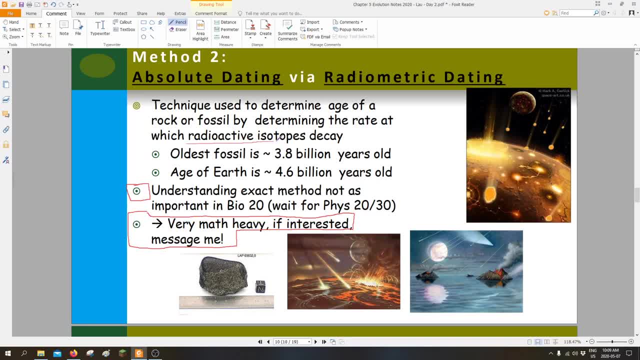 specific elements that are radioactive in your fossil samples and, doing a little bit of math, you can determine how old the fossil is. Some quick facts: the age of the earth is estimated to be about 4.6 billion years old. because of the way certain radioactive elements on the earth have 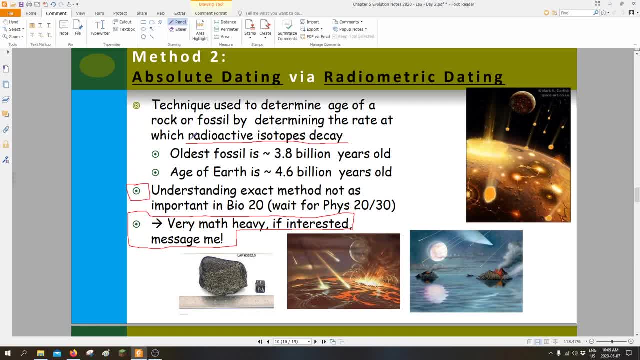 decayed over time or changed over time, et cetera, And the oldest fossil is estimated to be about 3.8 billion years old. again using these radioactive isotopes On the Google classroom, I'm going to link you one or two videos that explain a little bit more. 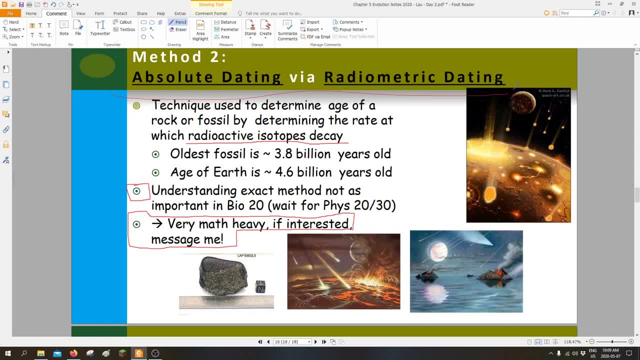 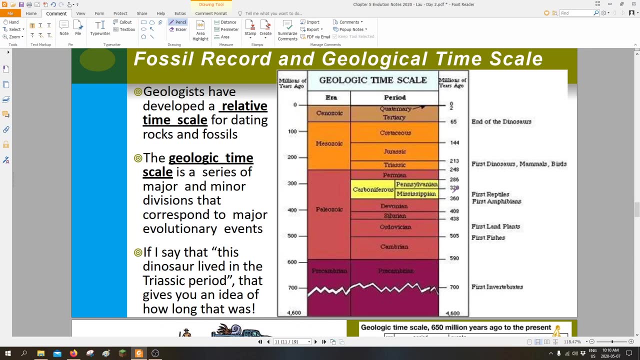 about radiometric dating, but you just need to know that this method exists. Do you need to know exactly how it works? No, If you want to know, you can ask me and I can definitely explain it to you. Okay, Now the fossil record and geological time scale. So when we talk about 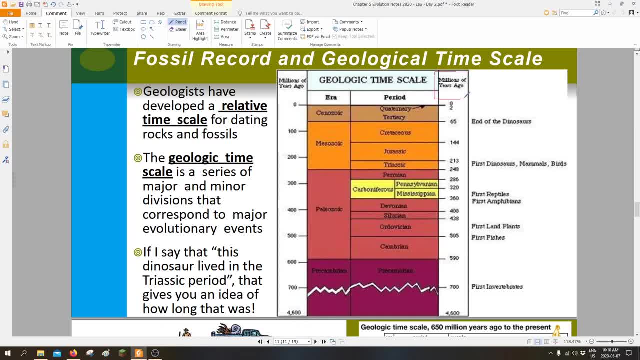 how old something is. we can't talk about how old it is in the millions of years, Okay. Or you can talk about it in a relative time scale, saying oh, maybe, like the end of the dinosaurs was right over here in the Cretaceous period, Okay, And if I tell you the Cretaceous period? 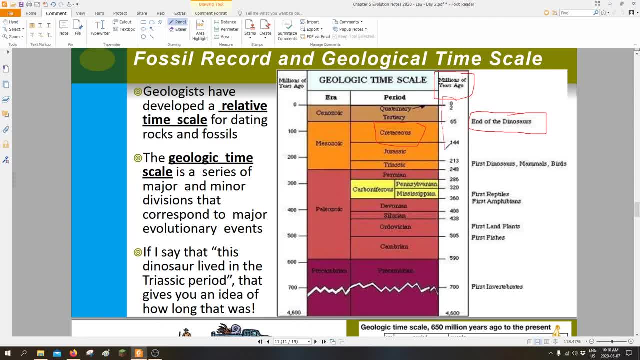 that gives you an idea of how old or how long ago that was. So the geological time scale is simply a series of major and minor divisions. okay, that correspond to major events. Some events are going to be very important in the evolution of the organisms. Some events are: 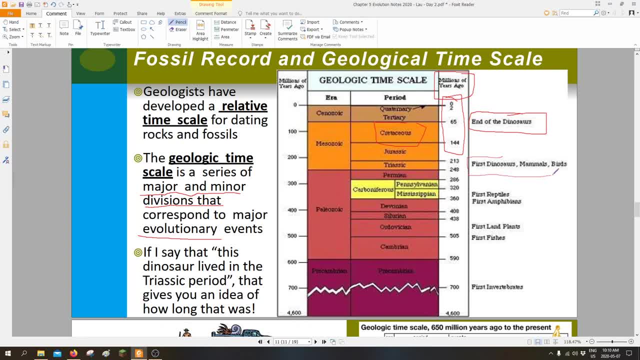 given to you. So, for example, dinosaurs, mammals and birds appeared evolutionarily during the Triassic period, about 213 to 248 millions of years ago. The first reptiles and first amphibians evolved about 320 to 360 millions of years ago or during the Carboniferous period over here. 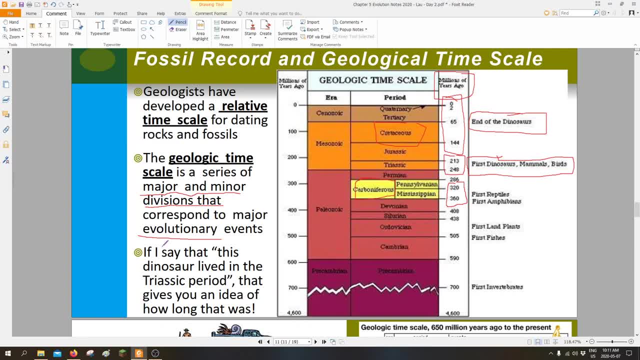 An example of how you use the geological time scale is if I tell you, oh, a certain dinosaur lived in the Triassic period, you already know how long ago that was simply by the words Triassic period. So there are certain eras that are very general, that encompass a lot of time, And then 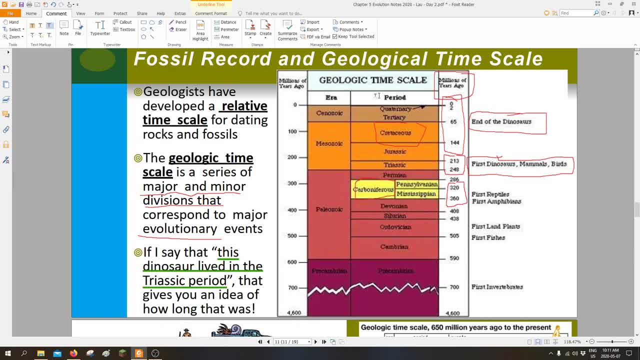 there are certain periods that are more specific and smaller in time as well. there We are estimating, or we're thinking, that the first intergalactic period is the Triassic period. So if I tell you that the first invertebrates- excuse me, the first invertebrates or organisms that had no spines, 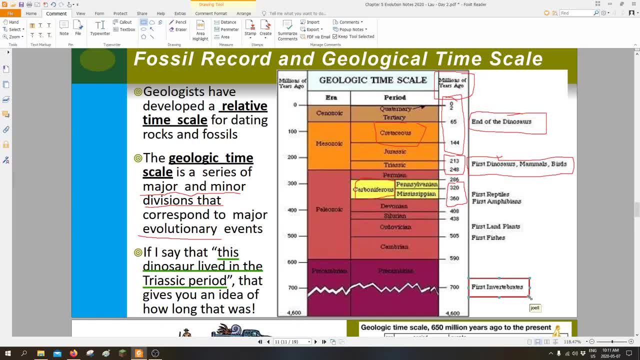 but are still like animals. they appeared about 700 million years ago. Again, these are just based in estimates, or instead of saying 700 million years ago, we can say the Precambrian period. Where do these all names? where do these names all come from? Probably from Latin or Greek. 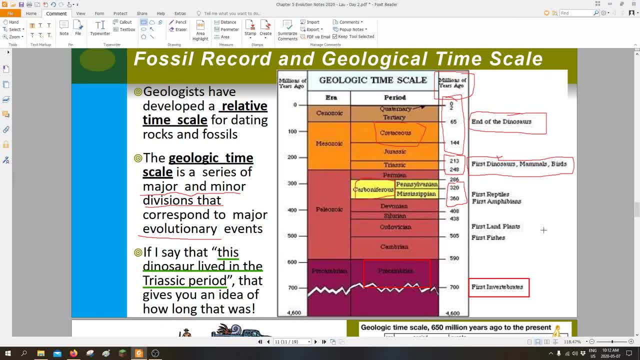 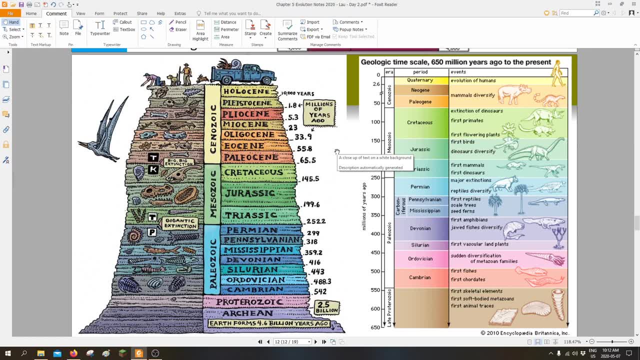 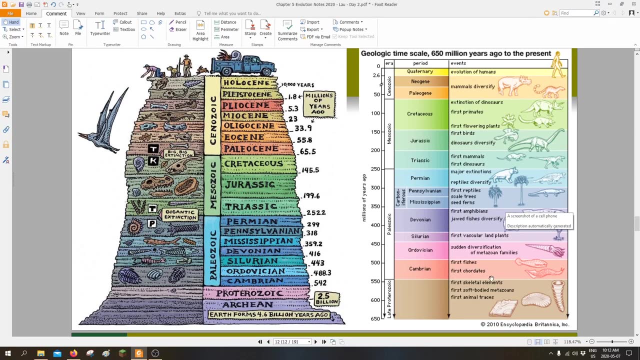 Again, we're not in a Latin or Greek class, but we just happen to use a lot of Latin and Greek terms. Here are two more pictures that are a little bit nicer looking and sort of give you an idea of what happened throughout time. Okay so, Cambrian period: first fishes and first chordates. 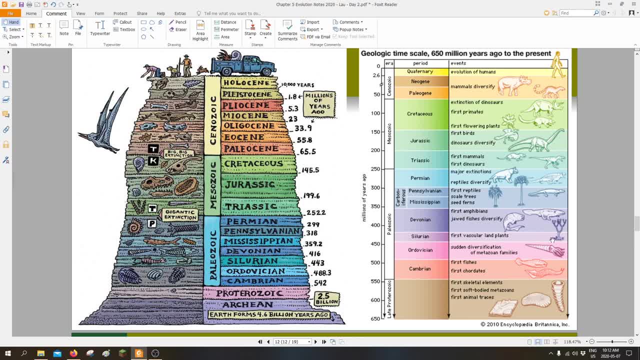 Okay, Silurian period. oh, the first vascular land plants. Okay, then mammals diversify in the Paleogean. a Paleo gene period? Okay, And again, when I talk about the Paleo gene period, I'm going to talk about the Paleo gene period. 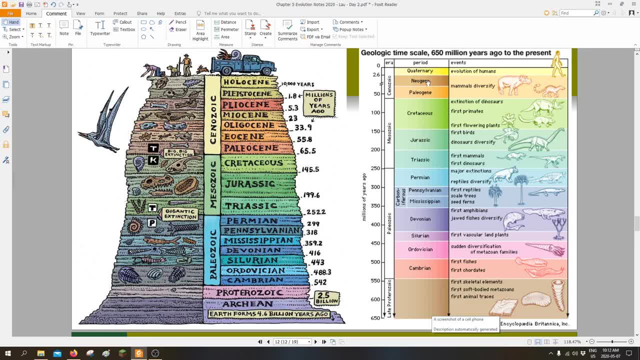 Okay, And again, when I talk about the Paleo gene period, I'm going to talk about the Paleo gene period. Okay. And again, when I talk about all these periods, I'm also talking about a particular time period in the millions of years ago frame there. 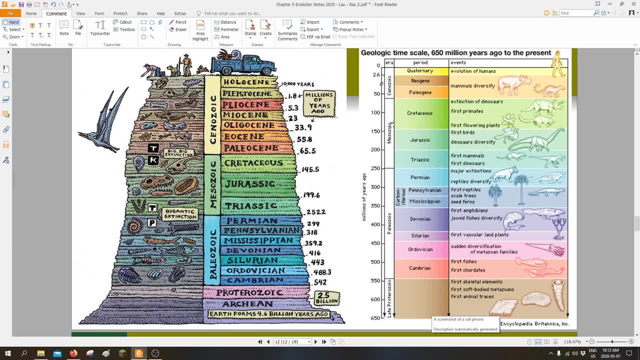 Cretaceous period about 100 years ago. Fun fact: the T-Rex. you might know this, but the T-Rex was not found in the Jurassic period. They're actually found in the Cretaceous period. I don't know why they call it Jurassic Park. It's frickin' Cretaceous Park. Okay, Also over here, there's another. Okay, Also over here, there's another. This is the Cretaceous period. I don't know why they call it Jurassic Park. It's frickin' Cretaceous Park. Okay, Also over here. there's another. This: 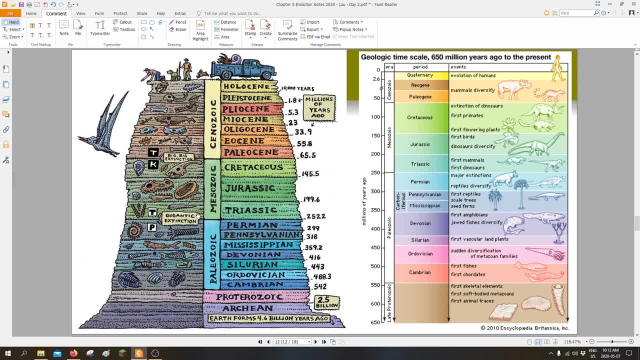 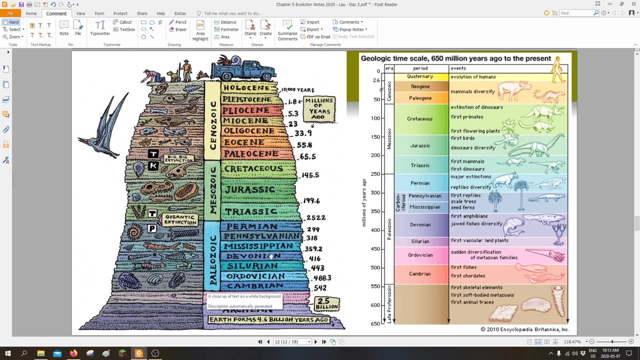 is the Cretaceous period. I don't know why they call it Jurassic Park. It's frickin' Cretaceous Park, Okay. Also over here there's another. This is the Cretaceous period. I don't know why they call it Cretaceous Park. It's frickin' Cretaceous Park, Okay. Also over here there's another. This is actually from a poster, actually. That sort of gives you an idea of the relationship between the fossils, the evolution of the organisms, the kinds of organisms that lived during these periods or millions of years ago in time, as well as a few different big extinction events. Okay, let's move on to the last part. 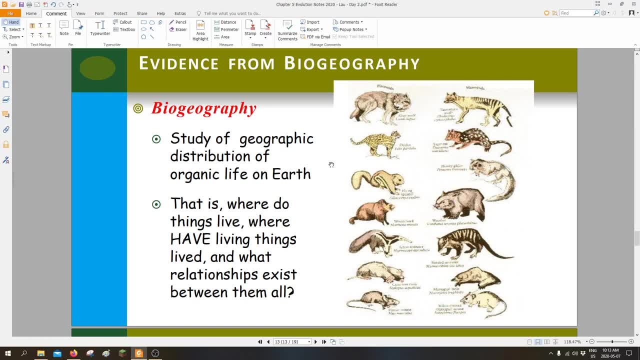 Okay, Let's move on to the last part. Okay, Let's move on to the last part. So we know what fossils are, we know how to figure out how old they are and we know how they show the evolution of organisms in terms of like the evidence that they have. 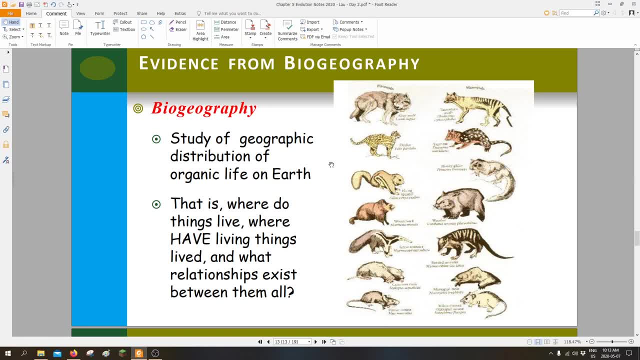 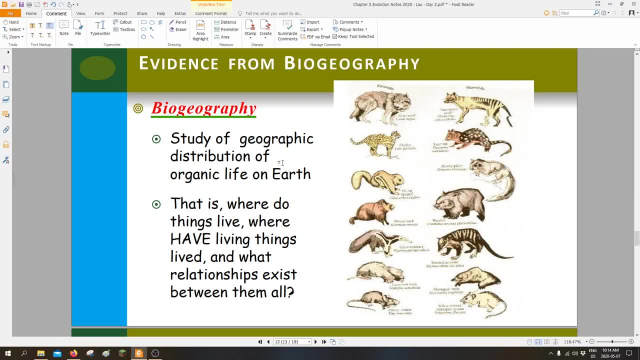 exist between what lives there and where they live. all of that's going to be related to biogeography as well. So, for example, it could be like: oh, where does this ocelot live, right? How is it different to where this anteater lives? And does where they live have any effect? 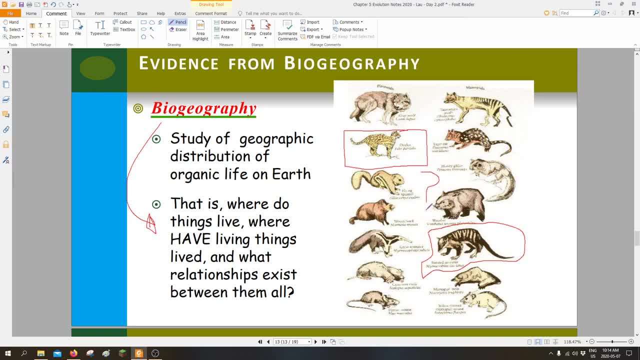 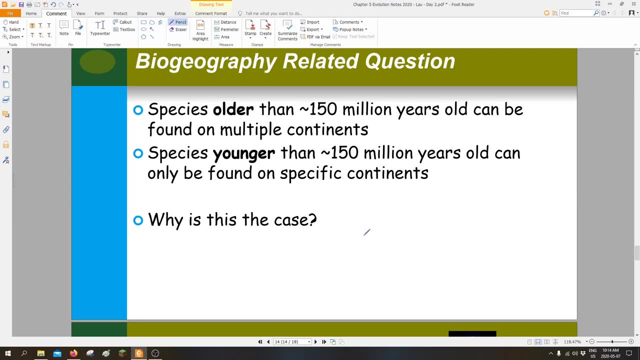 on their evolution, And that would be the question a biogeographist would probably ask. All right, So two questions that we would actually have to, two big questions that biogeographic biologists would have to take a look at, would be two questions. Number one: 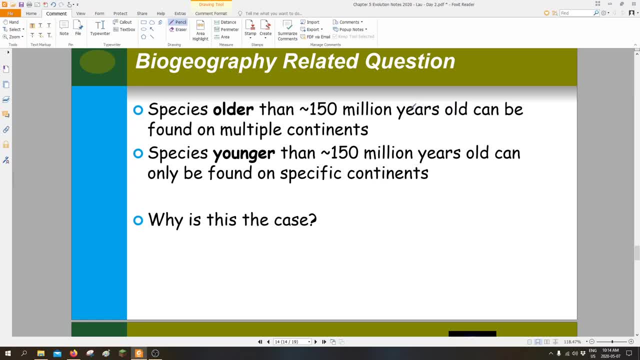 species that are older than 150 million years old seem to be found on multiple continents, but species that are younger than 150 million years old are only found on specific continents. Why is that So? the theory that biogeography, biographic, biogeography, biology- okay, A person who studies biogeography 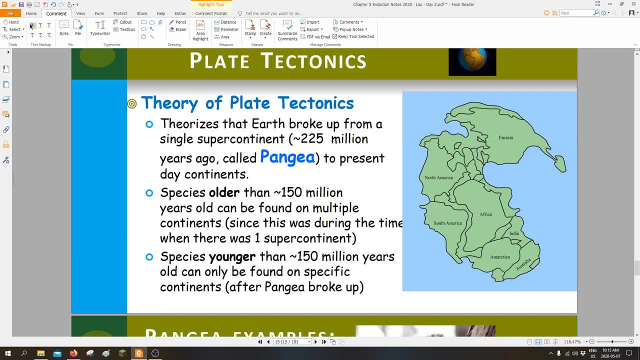 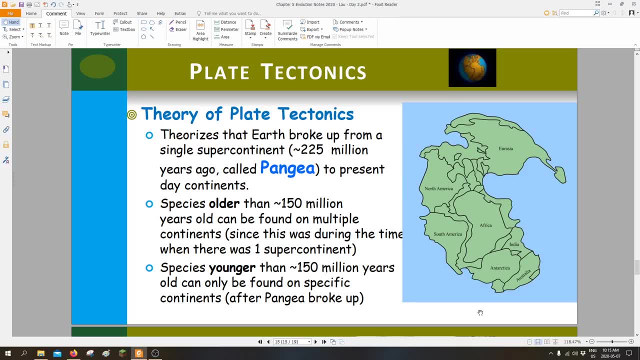 would be right over here, something called plate tectonics. You might have already heard about this before as well as you may have seen a picture related to this on the very first slide of this lesson here. So plate tectonics: we know that the earth's crusts and all the continents 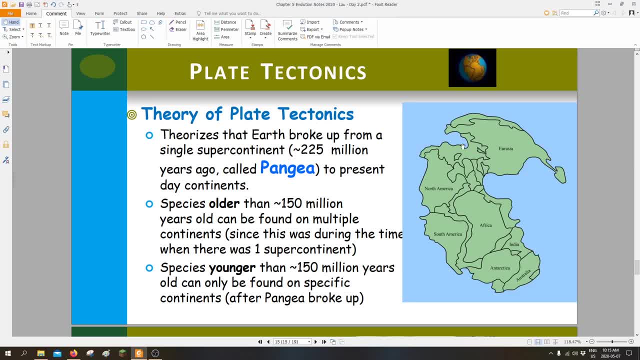 are separated on certain plates that can all move around on the earth. What biogeo biogeographers estimate or believe is that many millions of years ago, about 225 million years ago, all the continents were connected onto one supercontinent in the ocean. 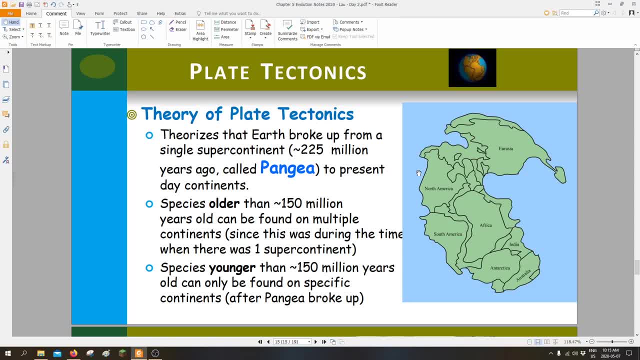 called Pangea. They called it Pangea. They, the humans 250 million years ago, didn't name it. It is just called Pangea by the scientists today. Many millions of years ago it used to be one supercontinent and the animals that existed here um. 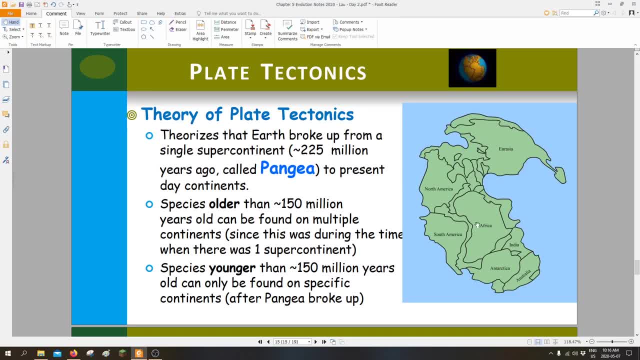 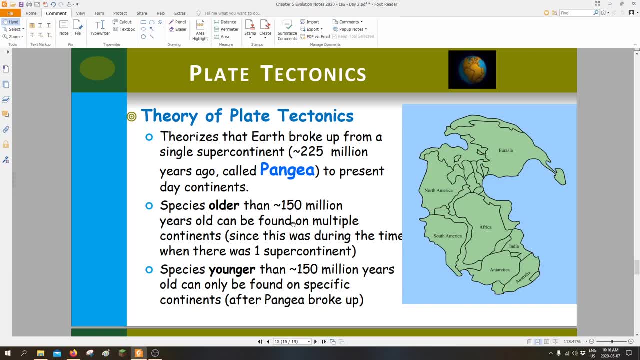 Eurasia, they could still walk and migrate to this part of Africa, this part of Antarctica, Australia, et cetera. And because it's all one supercontinent, okay, species that are older than 150 million years ago can be found on multiple continents, because they were all found in the 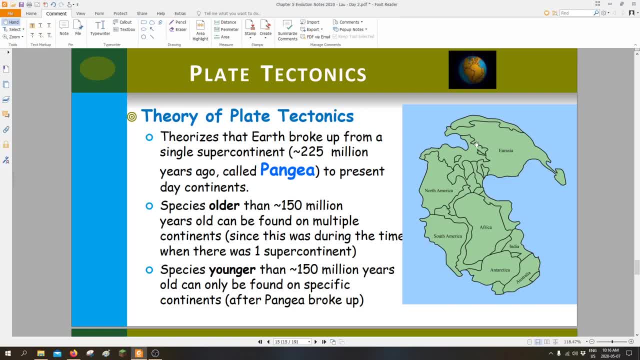 same area all along this supercontinent when it didn't break up. However, once they broke out, okay, once the Pangea uh broke up, and then evolution still went forward, okay. so, for example, let's say, um, let's say we have one organism that is going to be labeled Organism A. 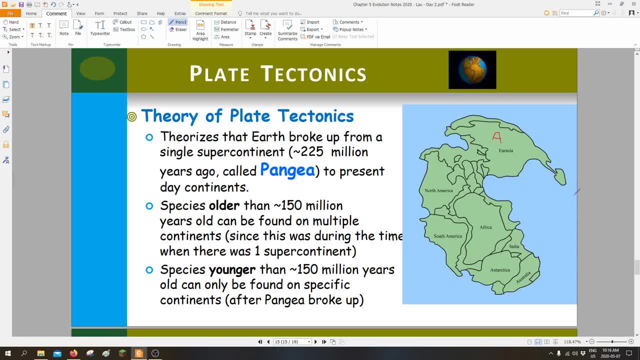 okay, Organism A lived during the time of Pangea. okay, So it can be living in this part. it can be living in this part. it can be living in this part. it can be living in this area as well. 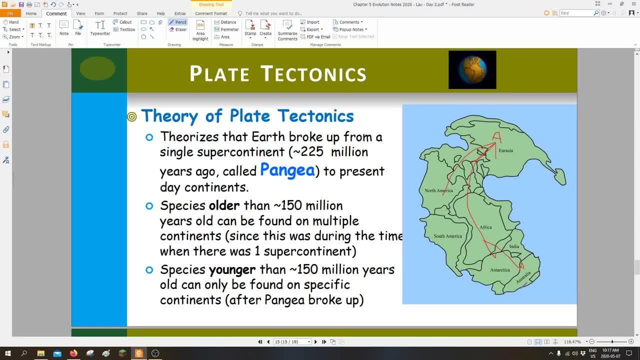 or Australia as well. there, okay, It can freely move around Pangea. okay, And then, once it broke out, once Pangea broke up, it could move around Pangea. okay, So it can freely move around Pangea. 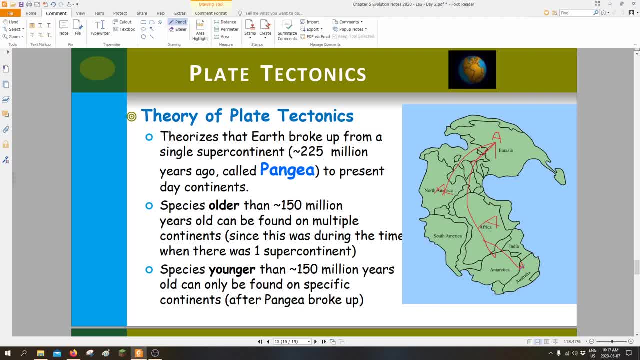 up. Well, you found A here, you found A here. you found organism A over here. Why? Because it could freely move all around before the breakup anyways. Now let's take a look at what if, once it broke up- okay, once Pangea broke up, okay, this is going to be separated. there, it's going to be separated. 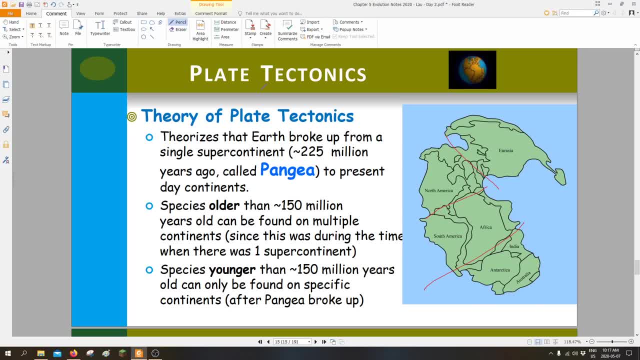 there, etc. If it breaks up. okay, if an organism evolves in Africa after Pangea broke up, well, guess what? This organism is only going to evolve in Africa. And after the breakup of Pangea- okay, is it going to be found in North America? No, because there was no way for this organism. 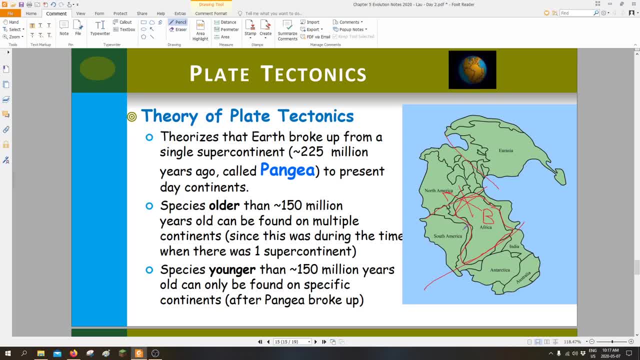 to travel to North America. there was no way for that to happen after Pangea broke up, So that is why we can say species that are older than 150 million years ago can be found on multiple continents, because it used to be able to travel everywhere on Pangea. 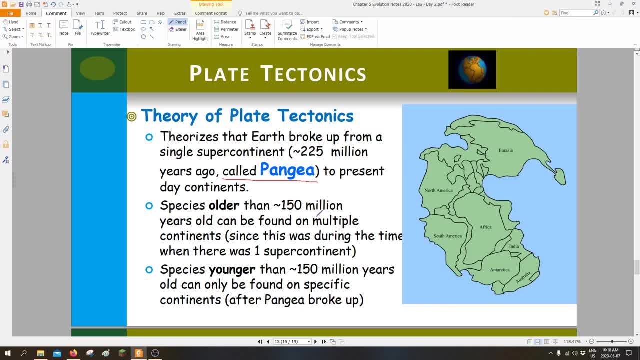 When all the continents were attached, But species that are younger than 150 million years ago can only be found on specific continents after Pangea broke up, because there was, there would be no way for them to travel across the different continents because all the oceans separate. 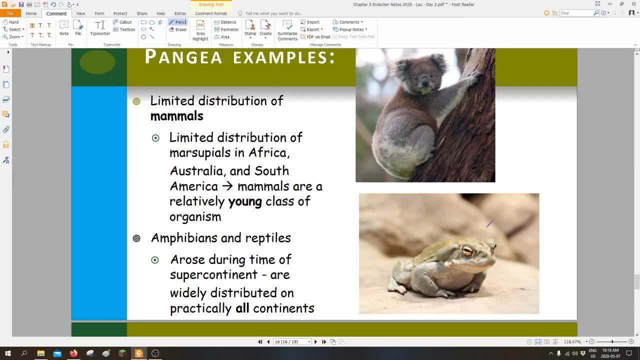 everything. Another example could be over here. Mammals are fairly young, okay, They didn't evolve until maybe a few million years ago, Okay, but amphibians and reptiles, in comparison, are very, very old. They are a class of organisms that are very old. 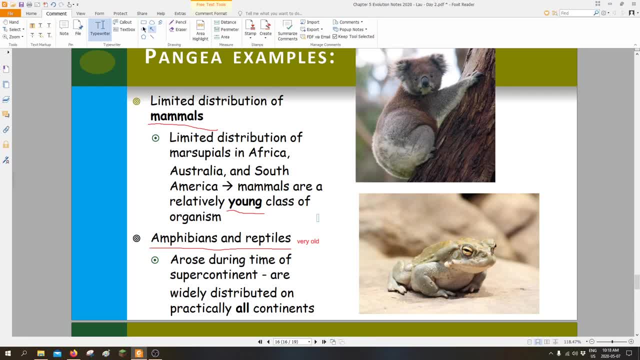 Because of that, they probably evolved during the time of the supercontinent, And if that's the case, they can be found all over the supercontinent. And once it broke out, well, they were just still on every single part of the continents, even after a broke up, So that is why you can find amphibians. 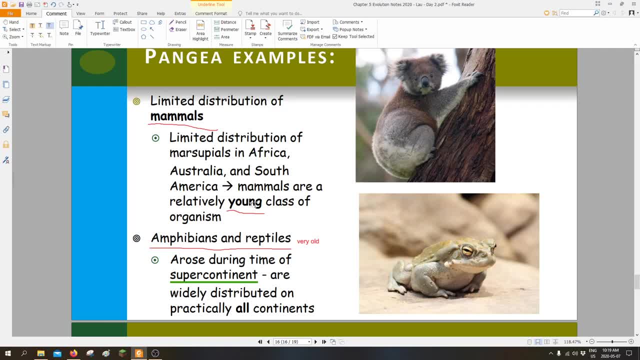 and reptiles in every single continent, And that's why you can find amphibians and reptiles in every- pretty much every single continent, But you can only find specific mammals in specific areas and in specific continents as well. What I mean by this class is, like you're not going to find a koala. 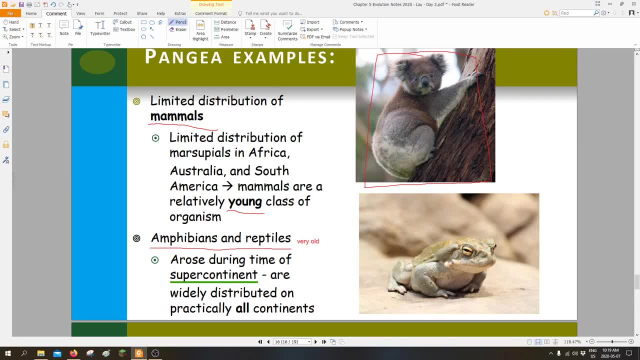 okay, you're not going to find a koala or any animal that's very similar to a koala in North America. Why? Because they evolved in Australia after Pangea broke up. However, you can find. you can find frogs that are very similar to each other everywhere. You can find them in Asia. 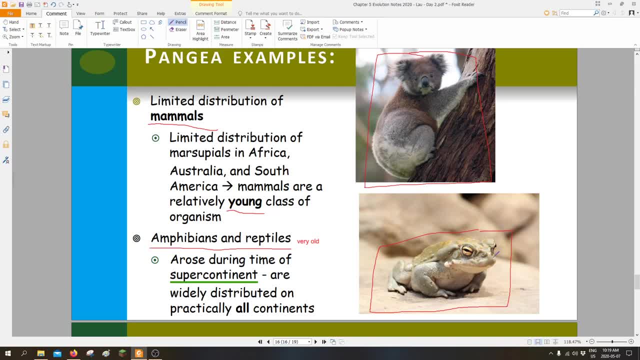 Australia, Britain, North America, South America, Central America, Africa. you can find frogs that are very similar to each other in every single continent, because their species is very, very old And they probably existed when Pangea did. Koalas did not exist during the time of Pangea And then. 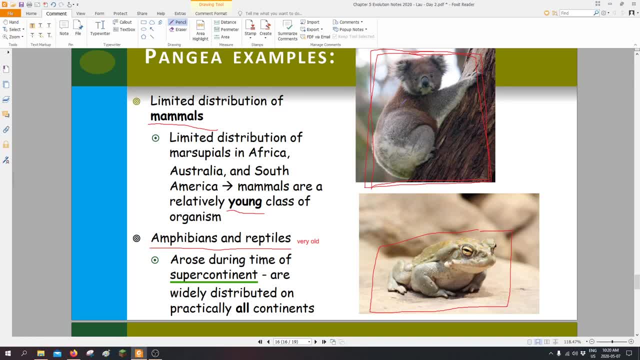 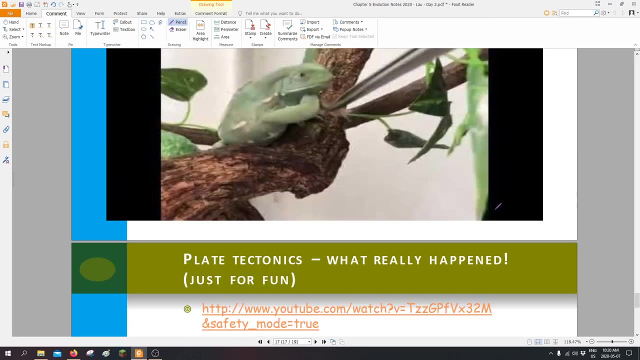 they only existed after Pangea broke up And after Australia became a waterlogged, or waterlogged by itself, And then, because of that, you can't find koalas anywhere else. All right, two videos. you can take a look at this one on your own, okay, And this is just a very 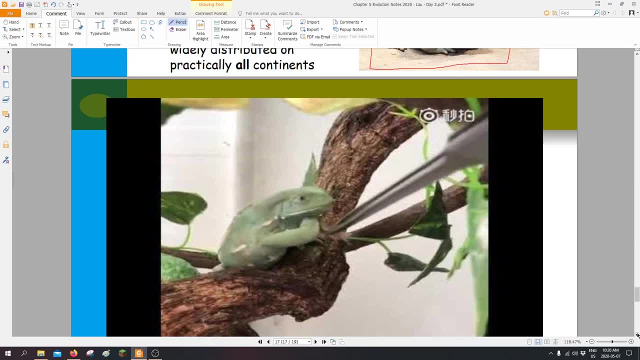 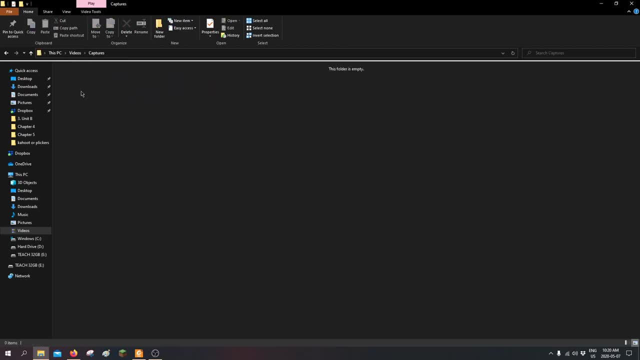 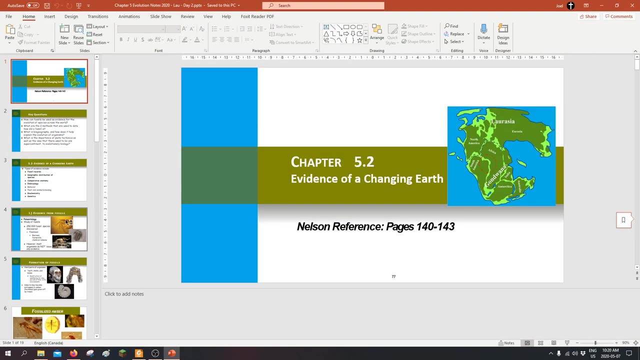 famous Facebook video of a frog denying a cricket that's being fed. I'm going to see if I can bring that up for you here. This is not the thing. Hold on, chapter five. hold on. Here we go. Okay, let's take a quick peek. Can I go like this? Oh, this is the wrong one. Hold on, wait, hold on. 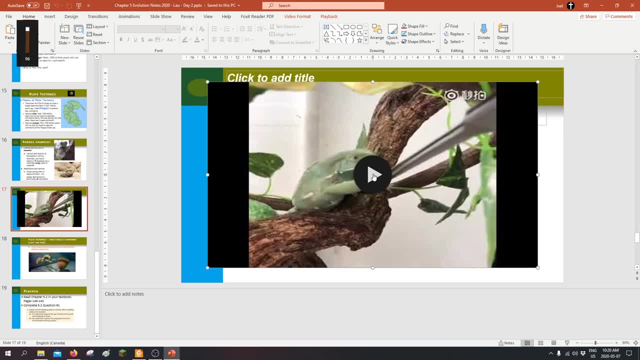 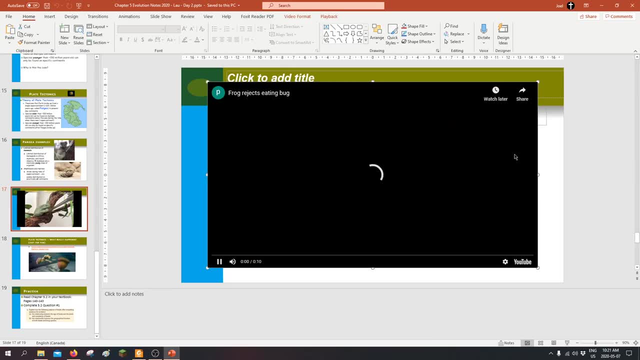 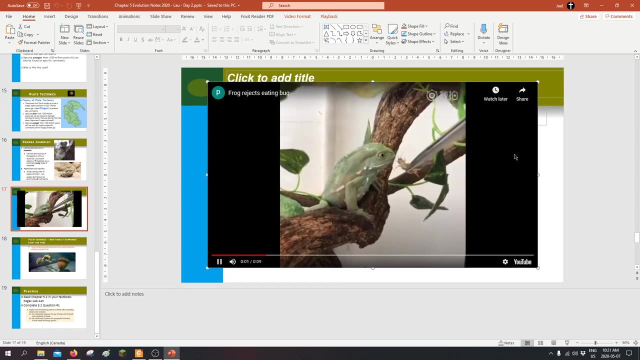 I'm just going to press this one. Okay, here we go. Let's take a look at this. Let's take a look at this. I don't think there's any sound. Hello, Is this working? Why, Here we go watch it. 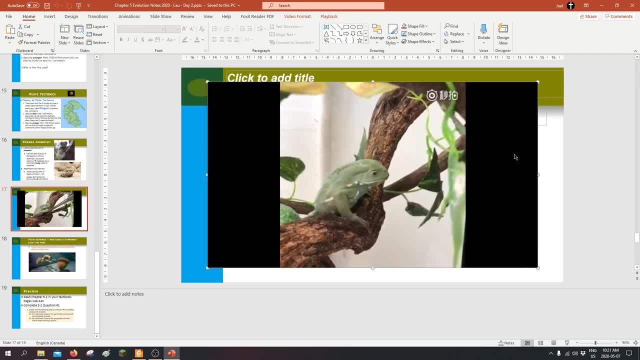 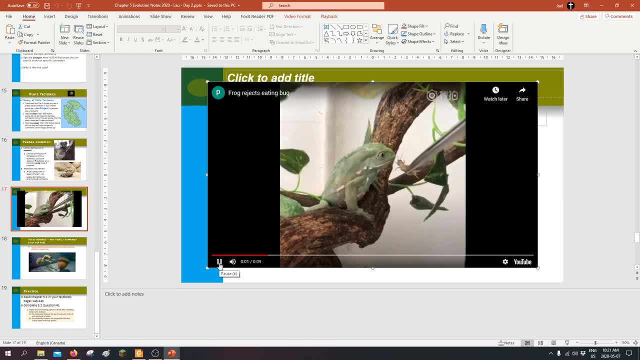 Watch what happens. Oh my gosh, that makes me laugh literally every single time, Like let's just watch it one more time. So I was like it's getting fed. It's like: what are you doing? I don't want to eat this. Hey, hey, get off of me. Hey, what are you trying to do? Get this out of. 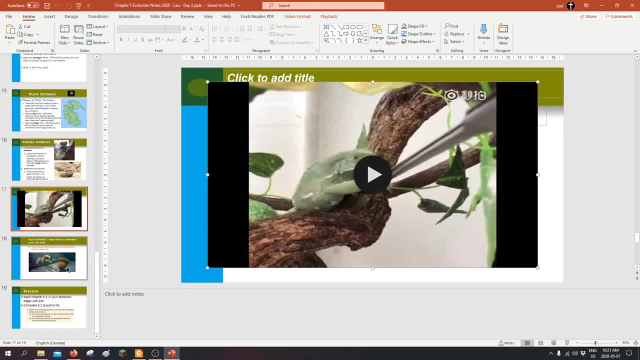 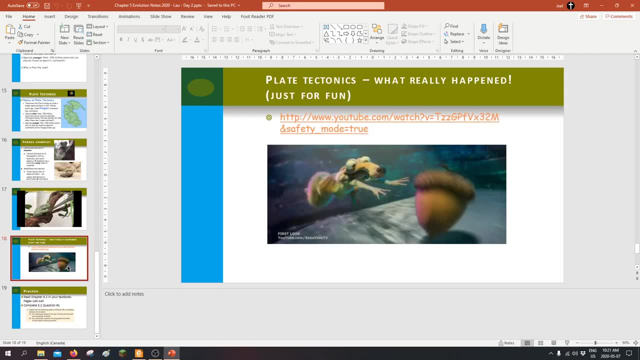 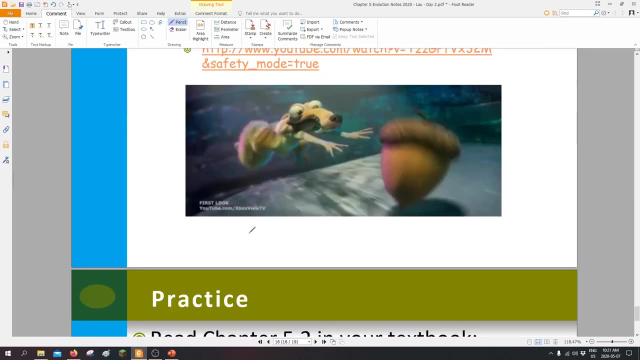 here. That's pretty funny. I love that video, It's great. And then this video over here is simply just a- what do you call it? A short little fictional adaptation of, oh, what really happened with Pangea, So you can watch this on your own, et cetera. Okay, last little bit over here, So that's.